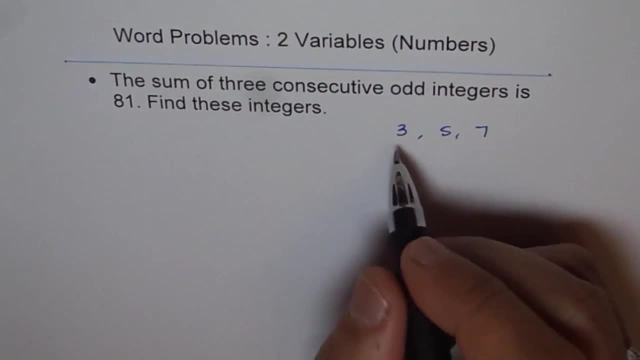 You will see a pattern. It is skipped by one. If I write value of 3, 5, 7,, it will be minus 3, 5, 7.. If I write value of 3, 5, 7,, it will. 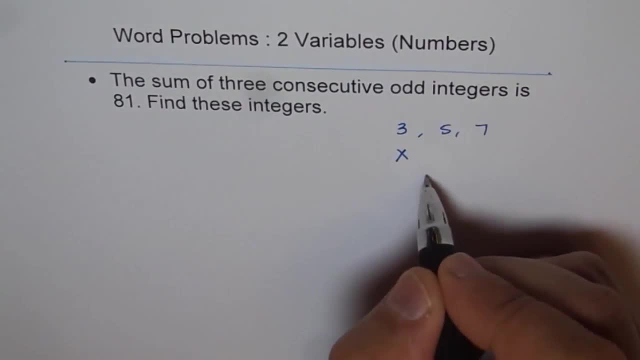 be minus 3, 5, 7.. If I write value of 3, 5, 7,, it will be minus 3, 5, 7.. If I write value of 3 as x in terms of variables, then what is y? I mean y. the next term is x plus 2.. 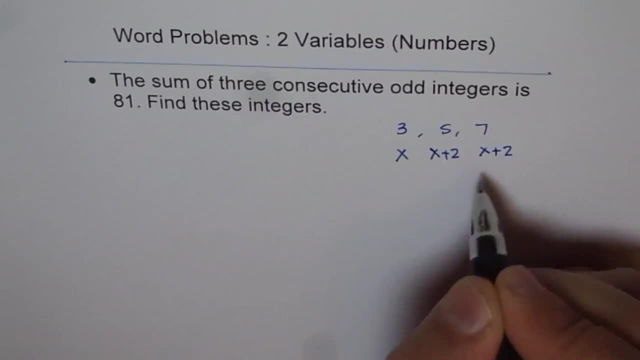 And then the next term you can get by adding 2 each time. So if you add 2 each time, then I should write plus 2, right, Add 2, more correct. So if you add 2 each time, you keep. 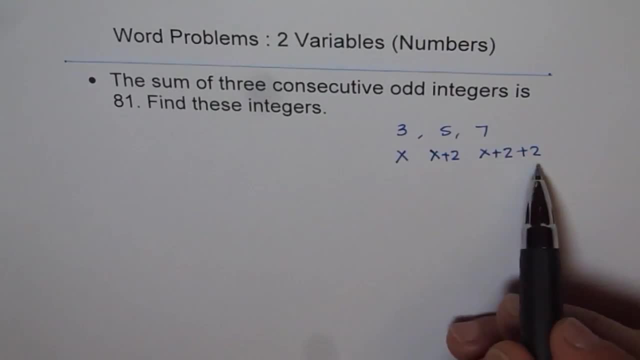 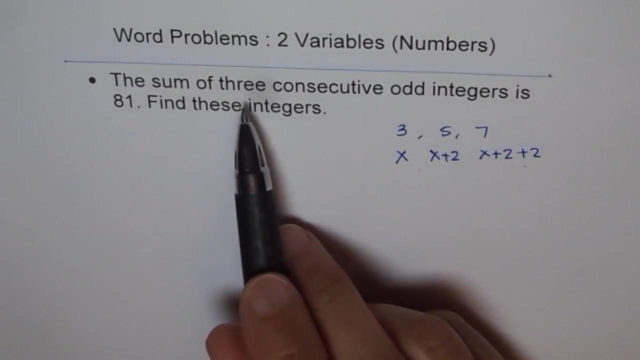 on getting odd integers in a sequence. So these integers in a sequence are called consecutive. So numbers which come in a sequence are consecutive numbers. So that is the basic understanding. So one way could be. you could say: 3 consecutive integers are x, y and z. 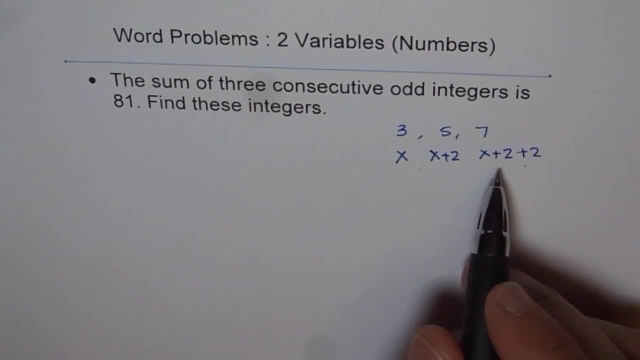 3 variables, Then the problem becomes very difficult to solve. So what we do is we treat it like this. We say: let So now I'll define the variables and you'll appreciate how we can define just one variable to represent 3.. 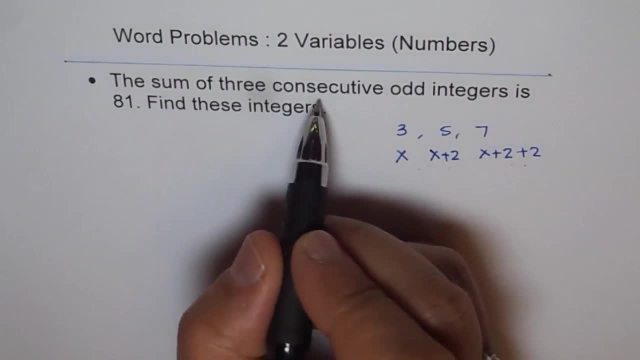 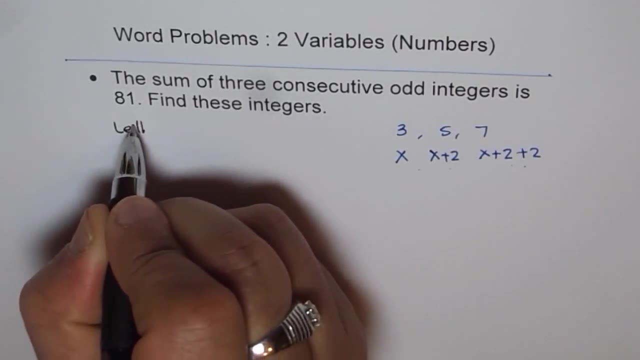 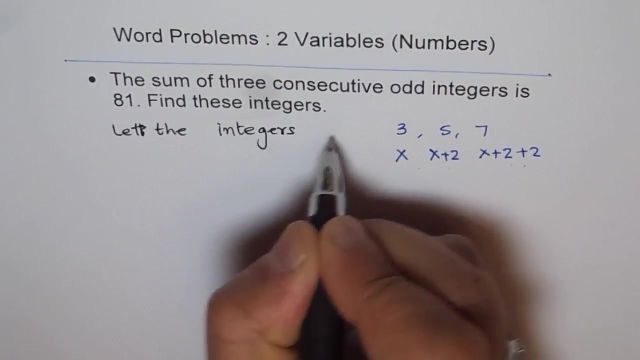 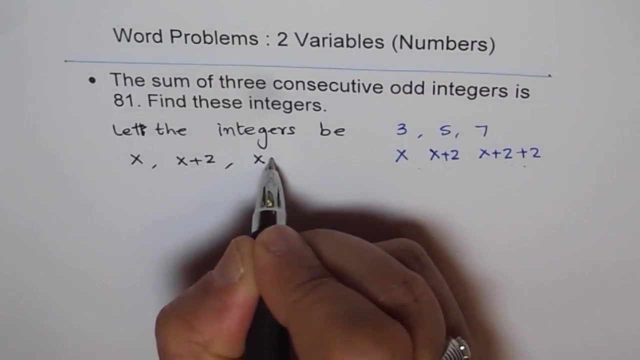 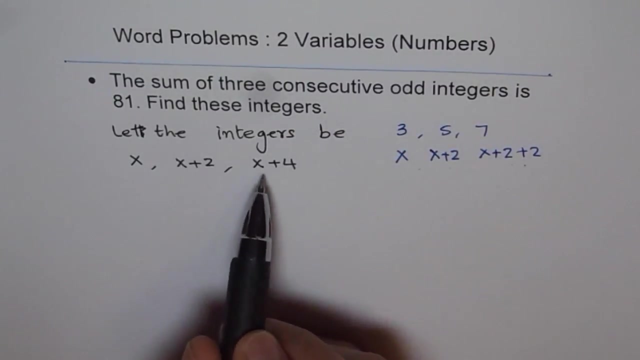 So it says the sum of 3 consecutive odd integers. So let the integers be x, x plus 2, and x plus 4.. Do you see this? If I write let the integers be x, x plus 2, and x plus 4,, I will get odd integers. Why did I add it too? Because I want to skip. 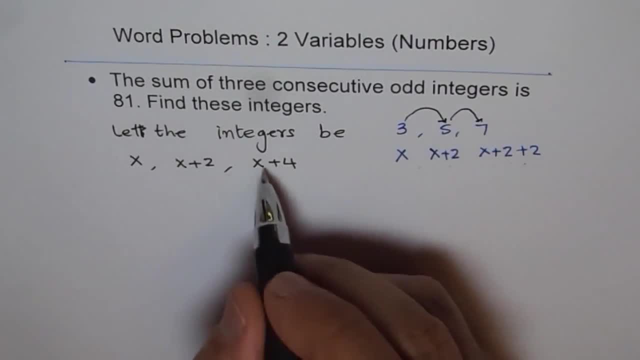 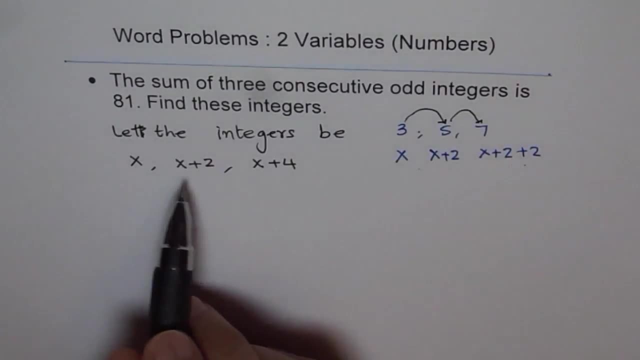 and get to the next odd number. If I write 1, I'll get the even number 4.. Do you see that I'm avoiding that? And the good part is that we are able to write this in terms of one variable, right. So that is. 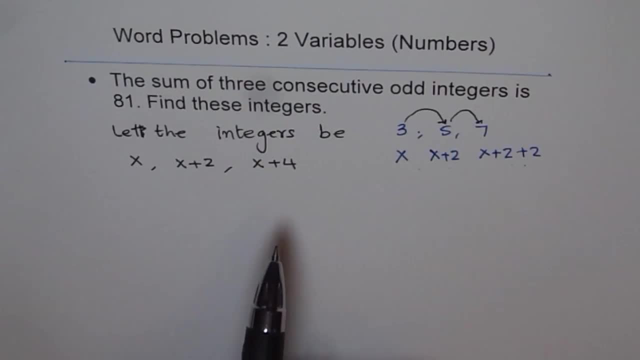 how we should define consecutive integers. Whenever you read consecutive integers, try to to put only one variable and then write your equation. okay, so the equation is: let the integers be x, x plus 2 and x plus 4, and that will give you the equation. read the problem once again. 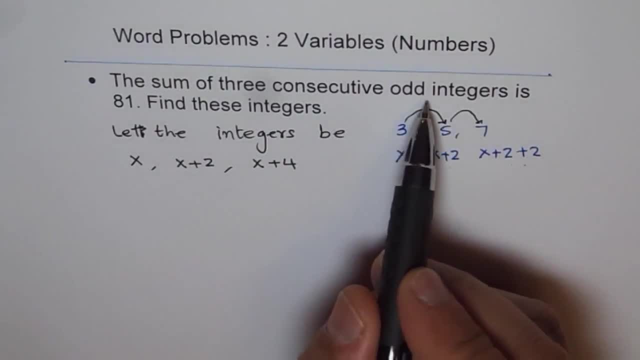 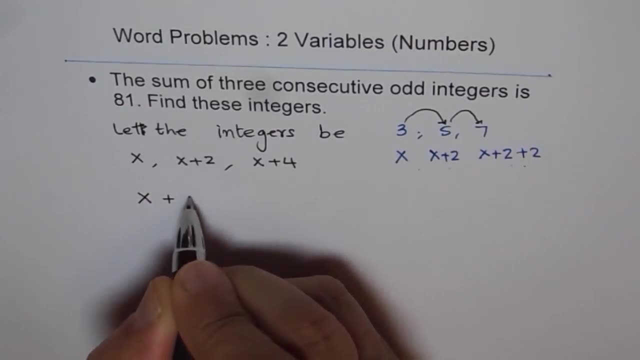 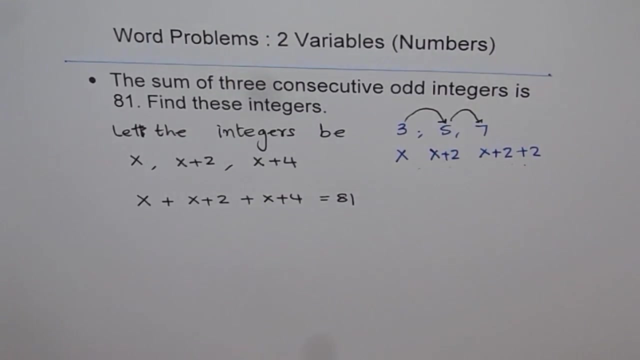 the sum of three consecutive order integers is 81, that is, if you add them, it should be 81. so let's add them and write down the equation: x plus x plus 2 plus x plus 4 equals to 81. so we got our equation. since there is only one variable- effectively it is x- one equation is enough to 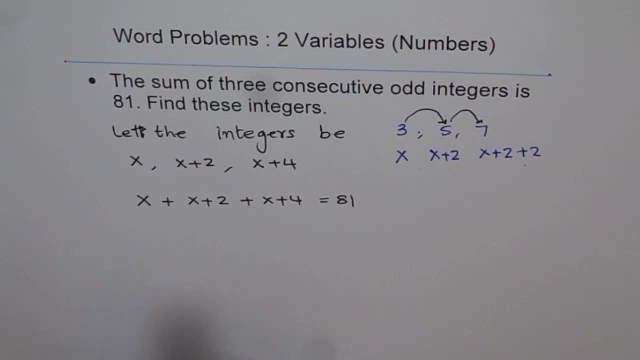 solve how many x's we have in this equation: 1, 2, 3. so we can write: 3x plus 2 plus 4, 6 is equals to 81. so we can rearrange and write: 3x equals to 81 minus 6, so we get which is equal to, we get: 3x is equals to 81 minus 6 at this stage. 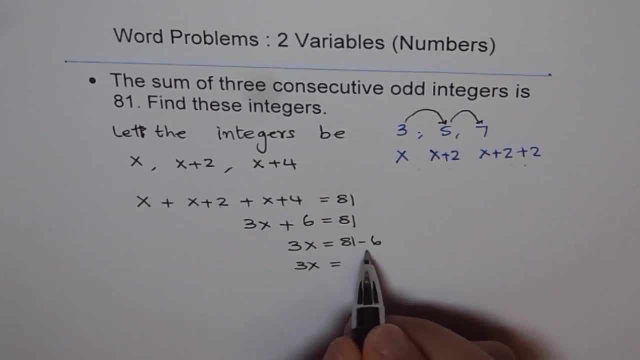 you can use the calculator also, right. so we get 81 minus 6 as 75. and from here you can say what is x? divide by 3, both sides, you get x equals to 75. divide by 3, right, which gives you 25. you. 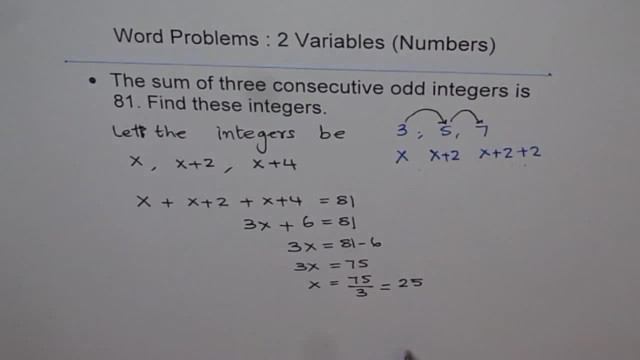 you 25, so x is 25. therefore, our integers will be: check your answer: 25, right? so x is 25, so x will be 25, x plus 2 will be 27 and then plus 2 will be 29. so these are the three integers for us, right? 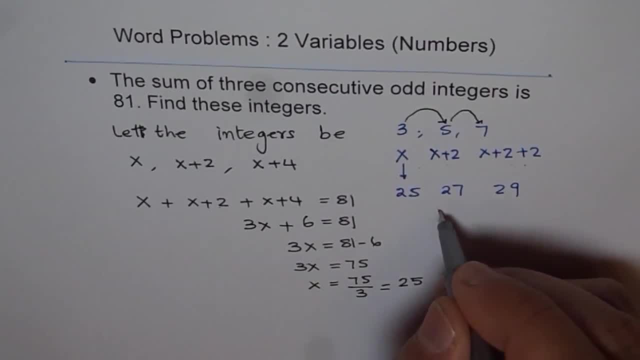 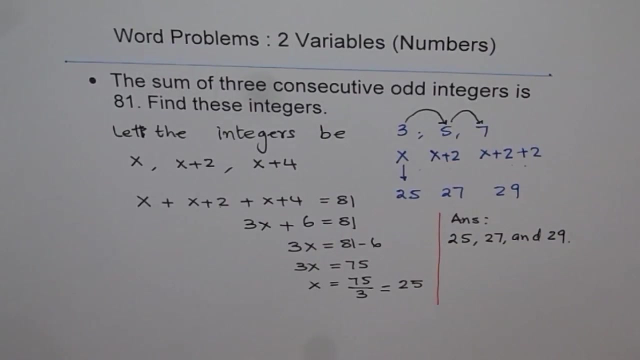 and therefore now you can write down your answer very clearly. right, let me write down the answer on this side and say: answer is like: the three consecutive odd integers are right, all that. okay, then like 25, 27 and 29, so that becomes your answer. right? you can add them at this stage and check. 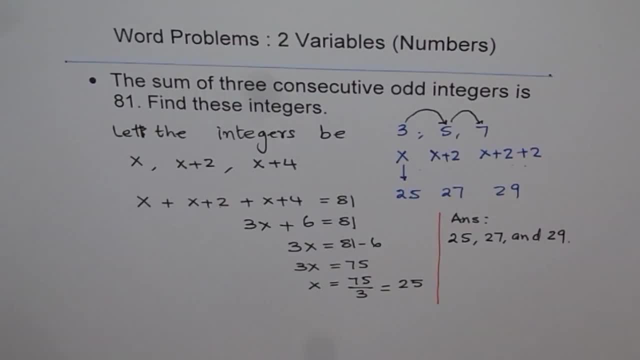 is the sum really 81. so check your answer. that is what i'm always saying: check. add them up, right. so 9 plus 7, 16 plus 5, 21, so you get 1 right. you had 2. carry forward 2 plus 2, 4, 6 and 8. that is right.